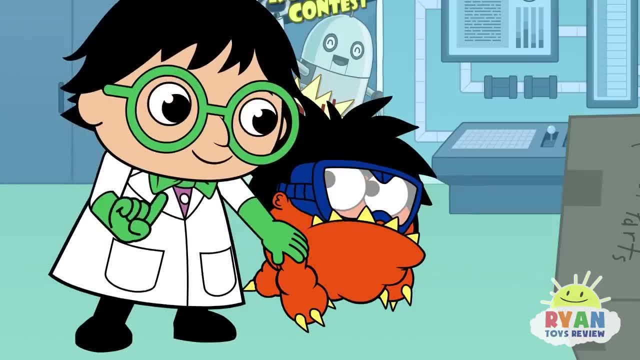 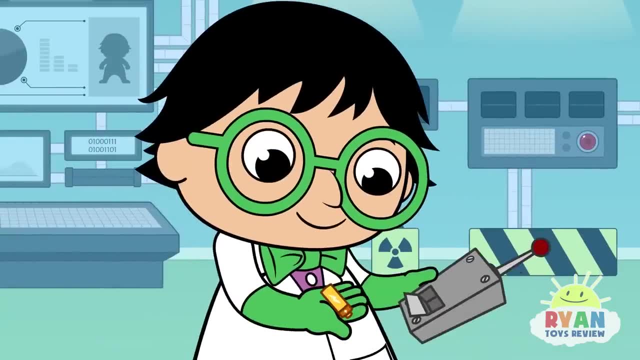 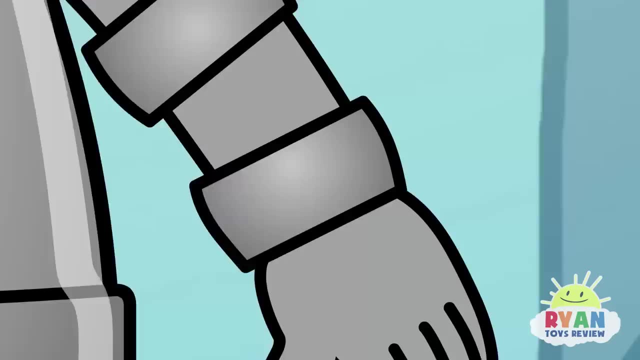 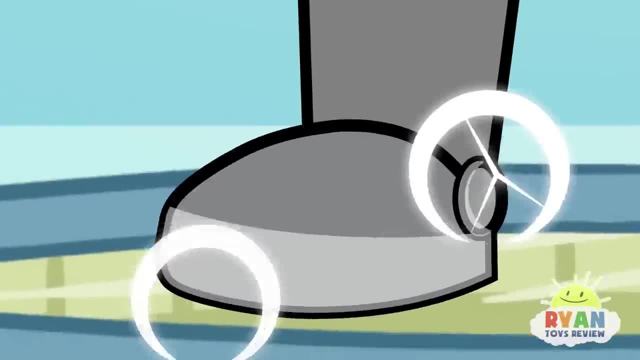 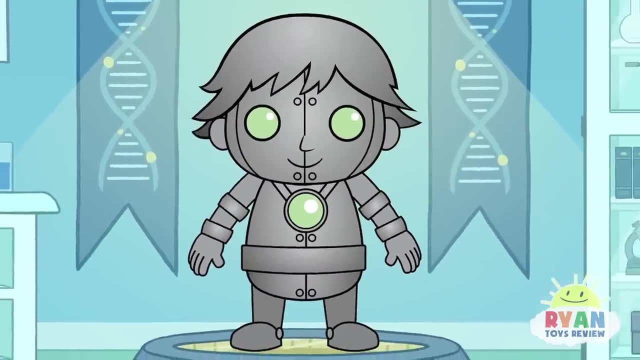 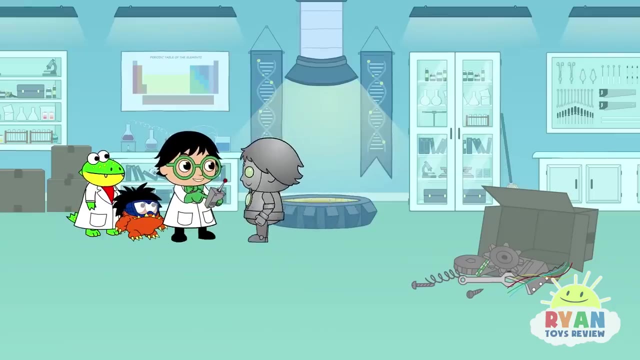 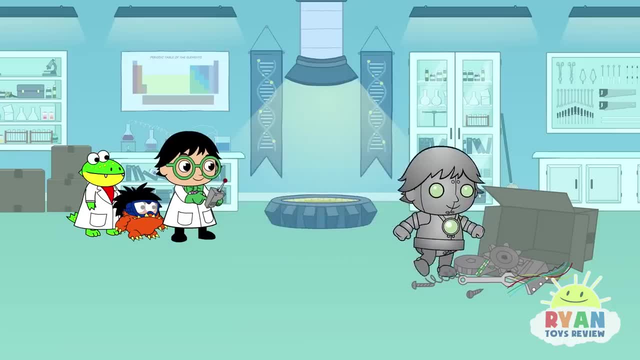 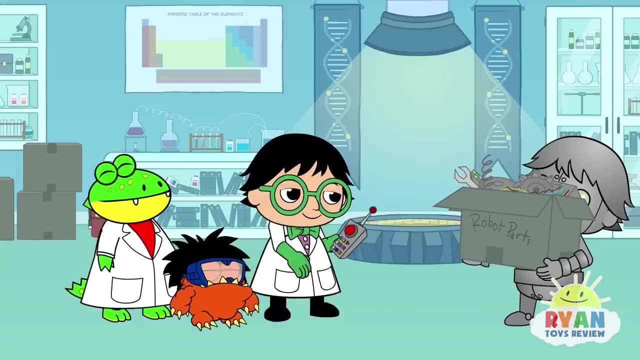 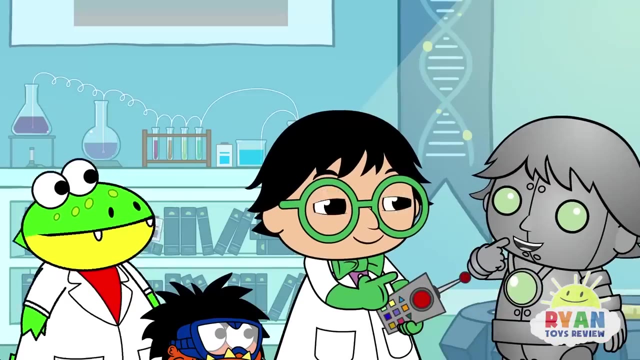 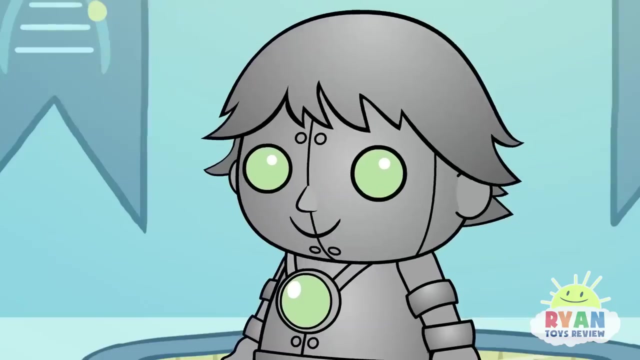 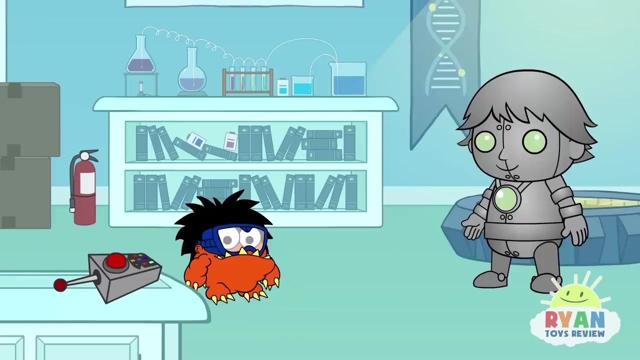 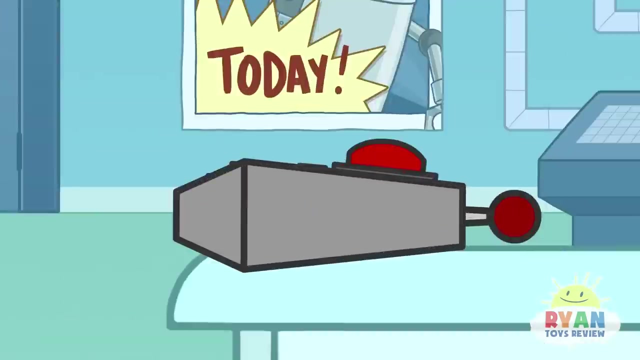 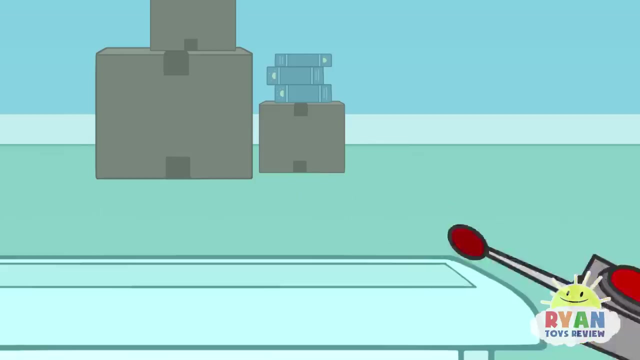 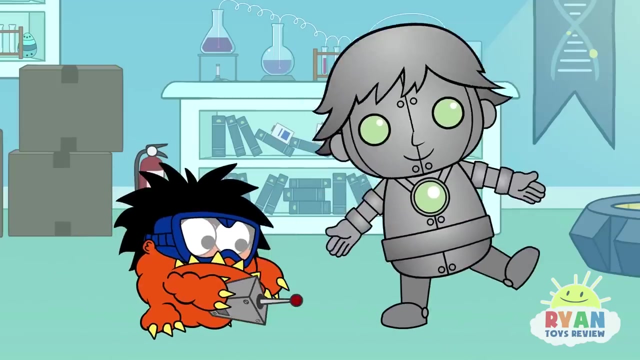 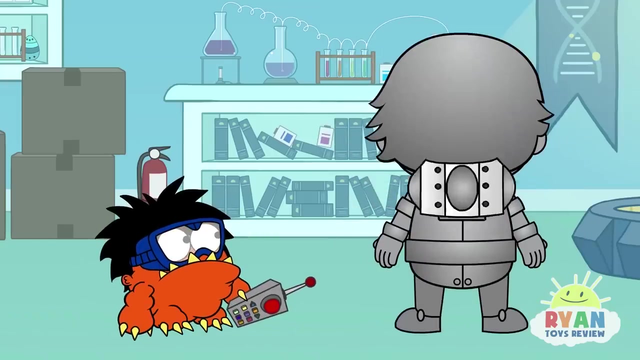 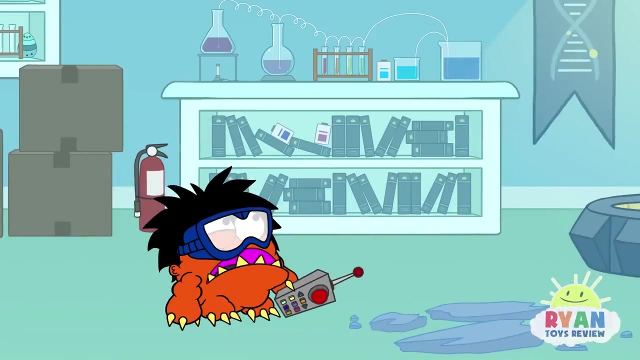 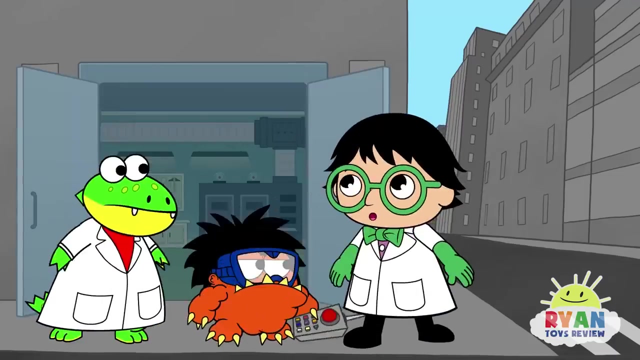 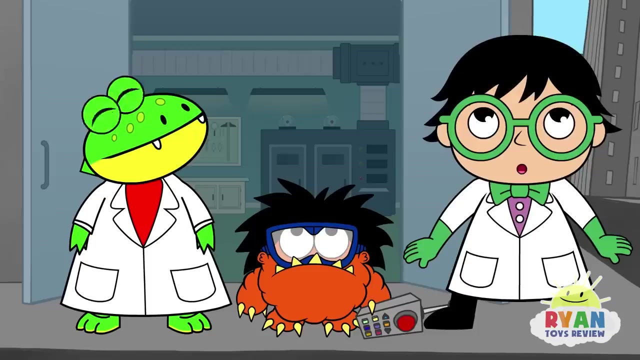 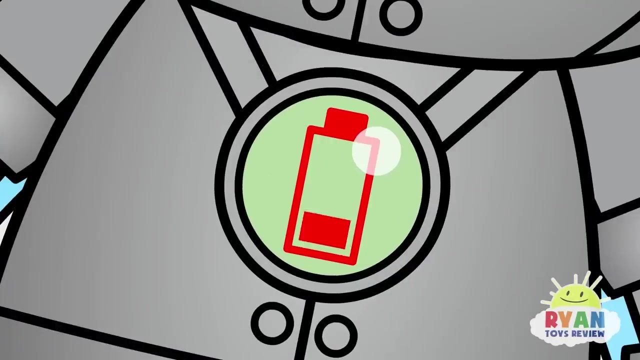 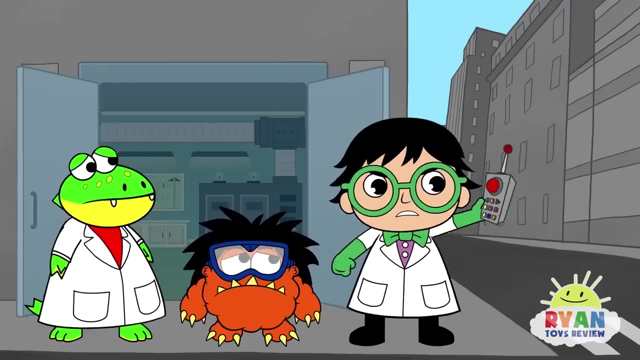 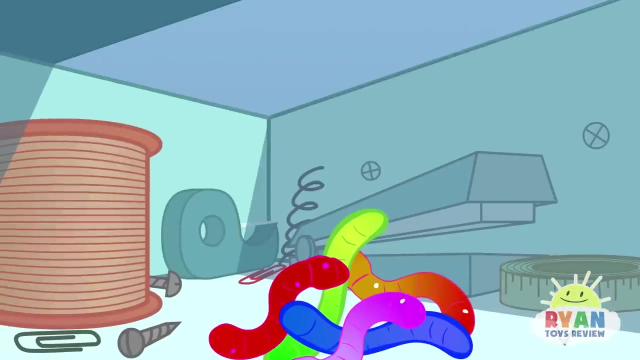 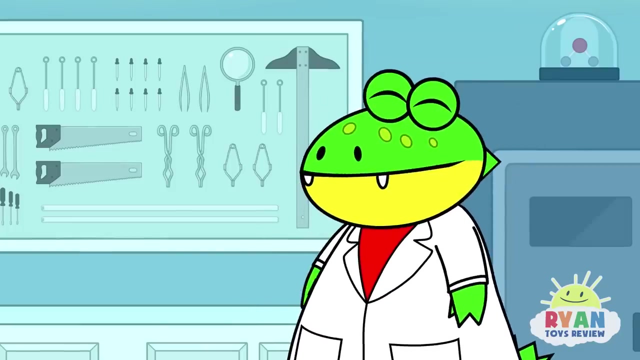 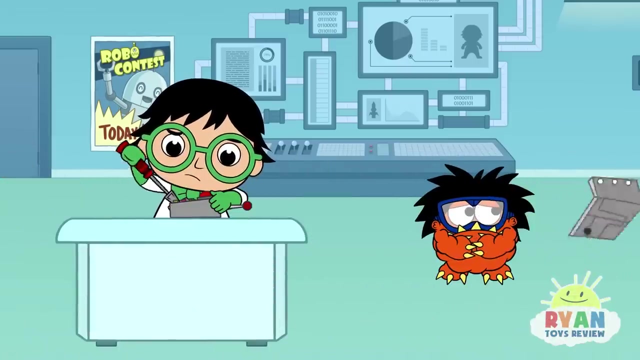 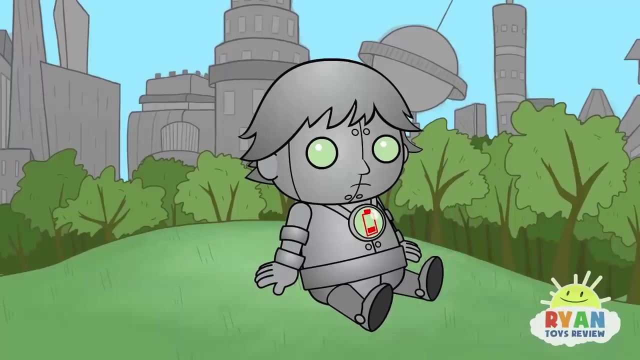 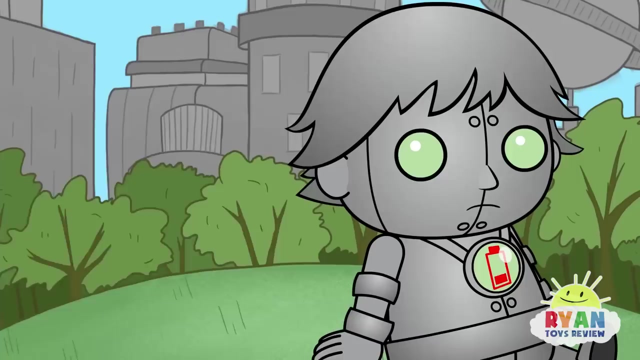 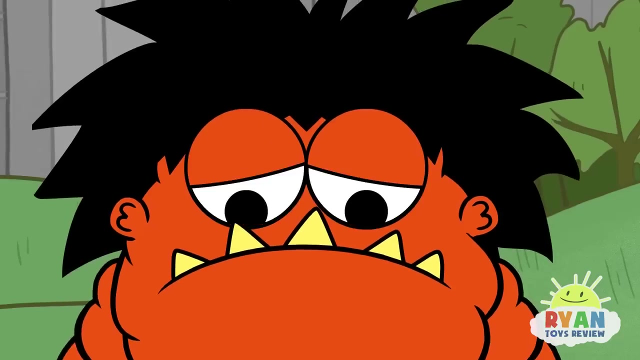 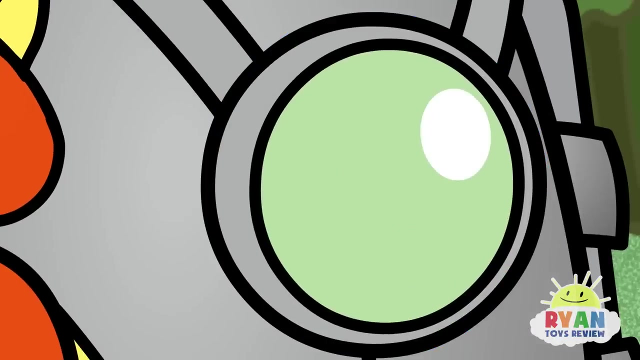 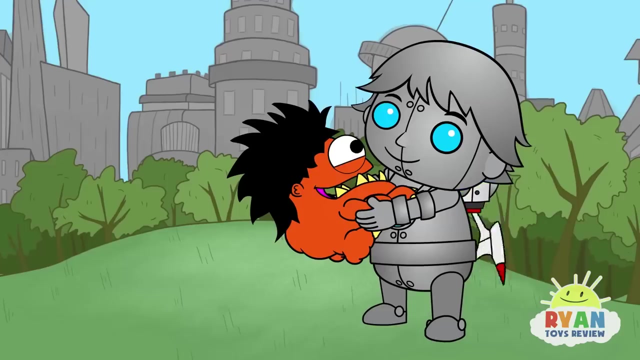 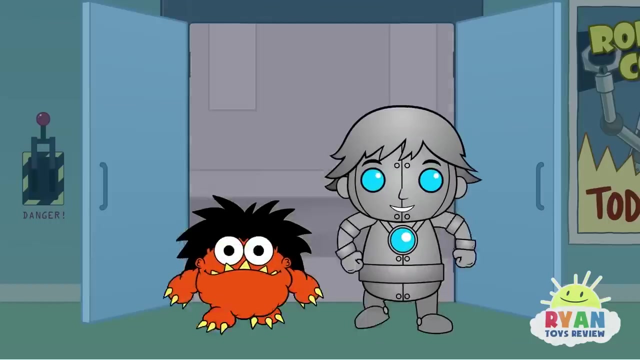 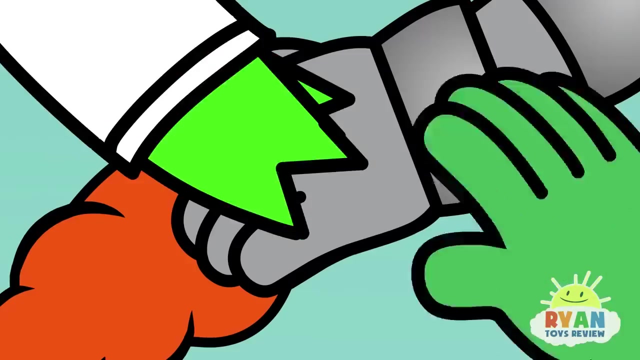 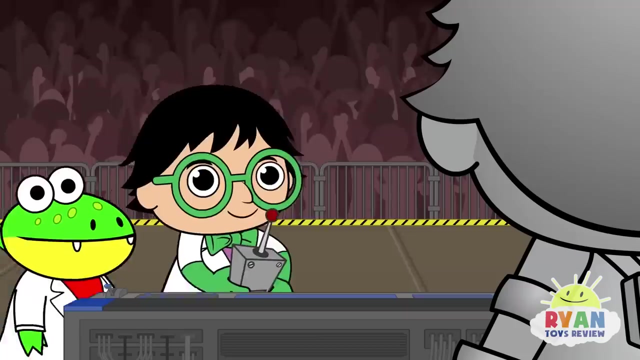 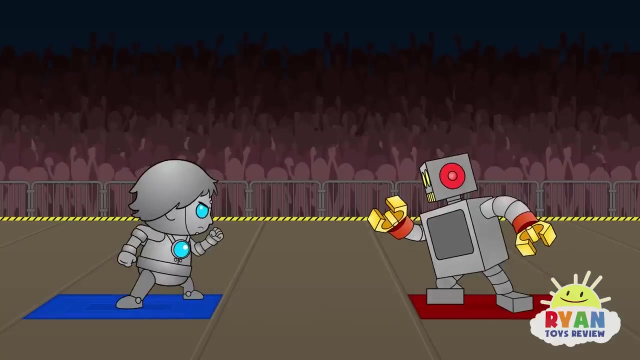 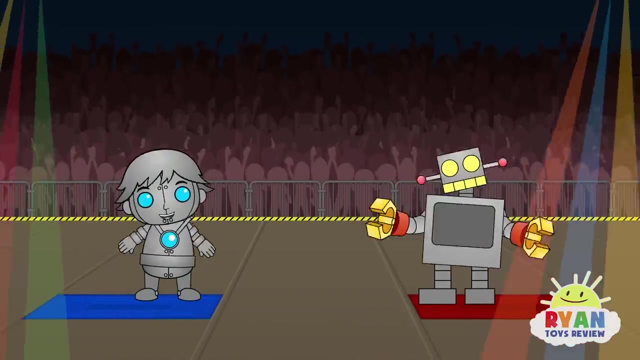 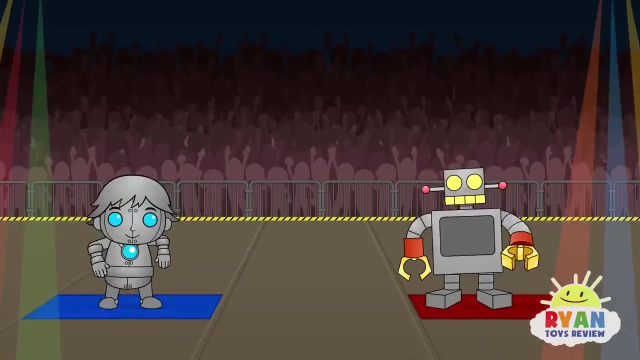 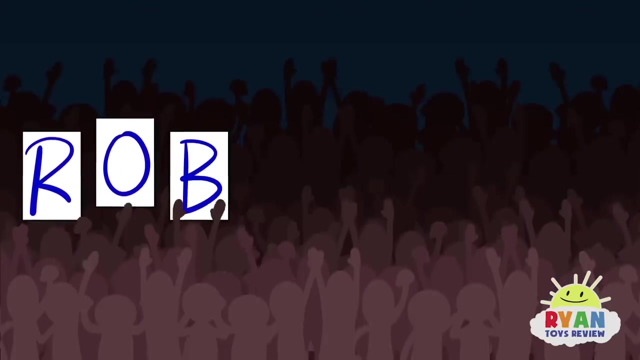 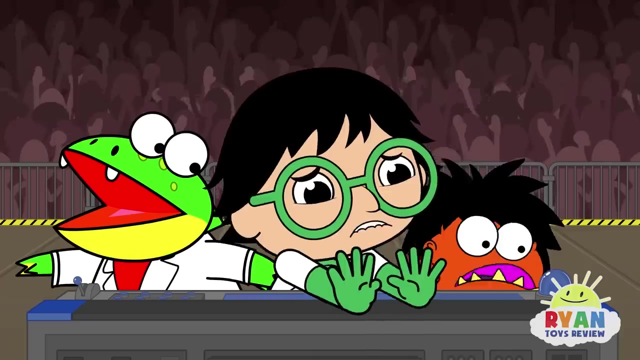 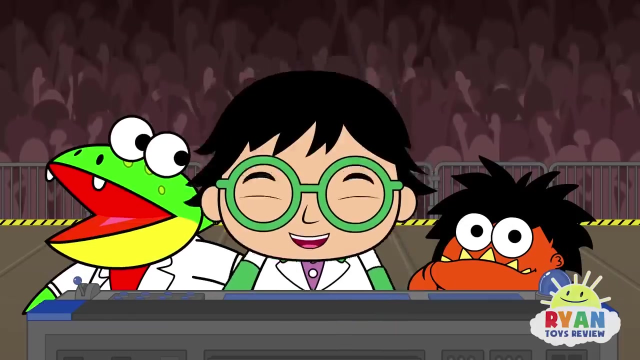 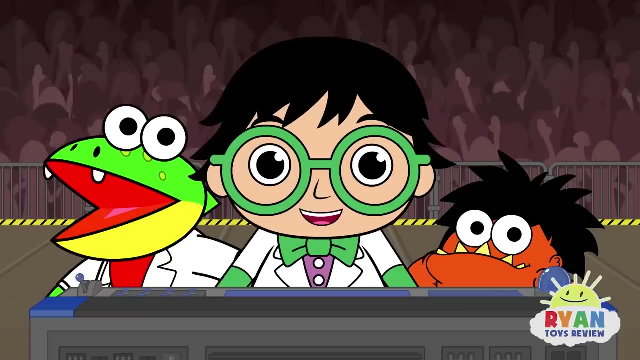 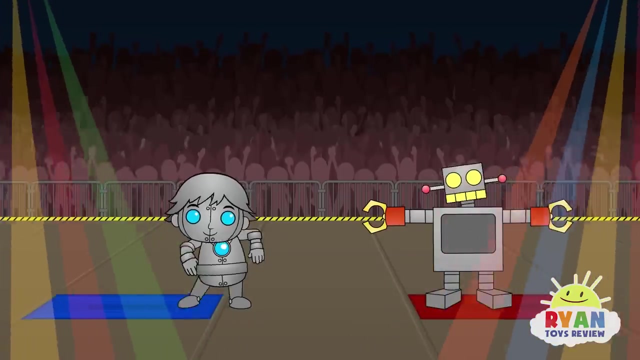 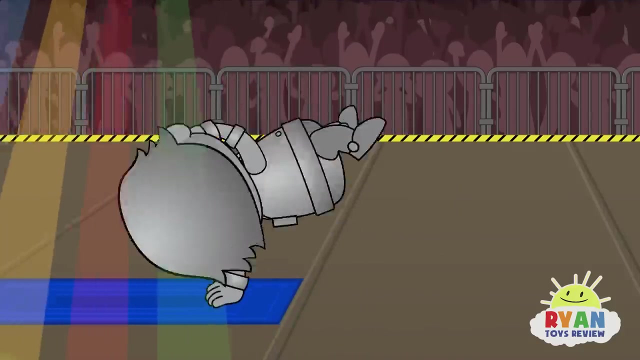 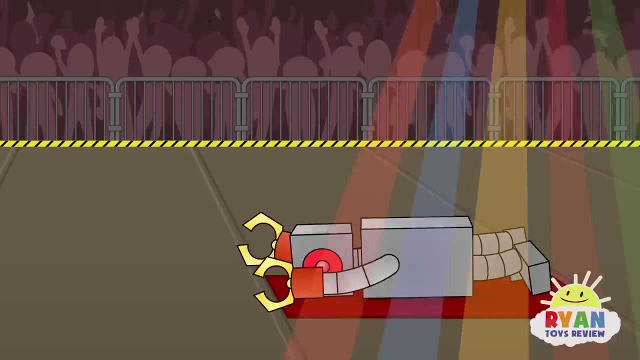 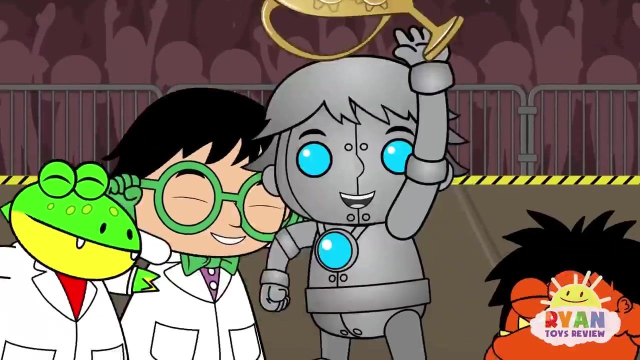 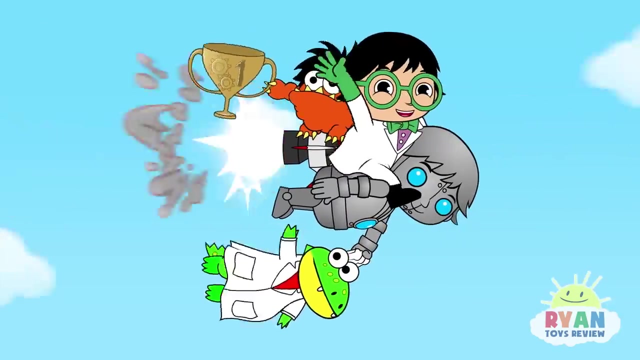 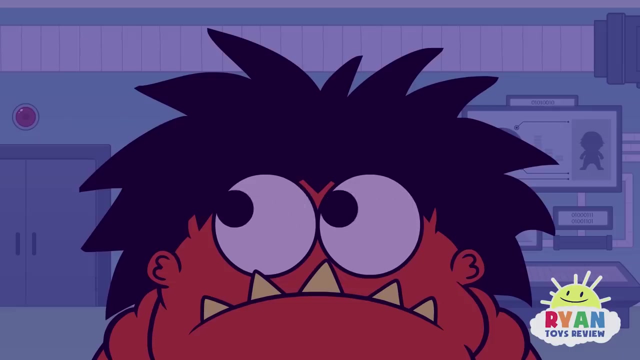 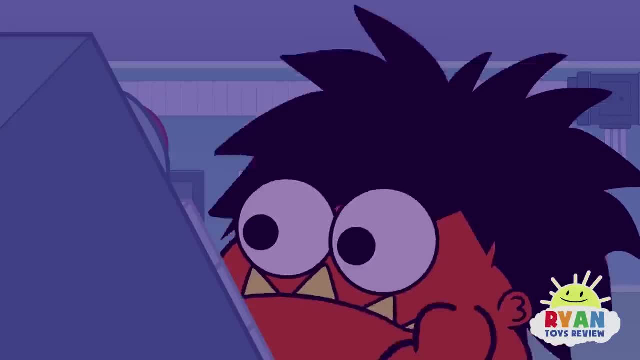 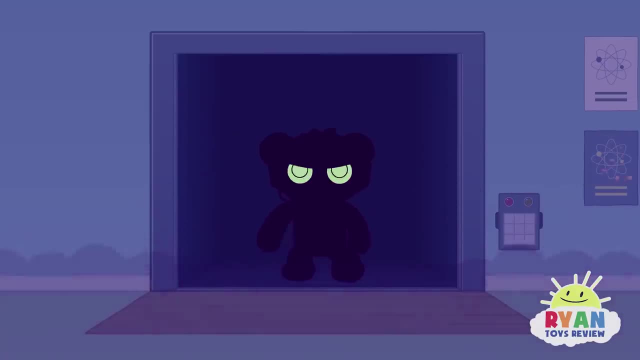 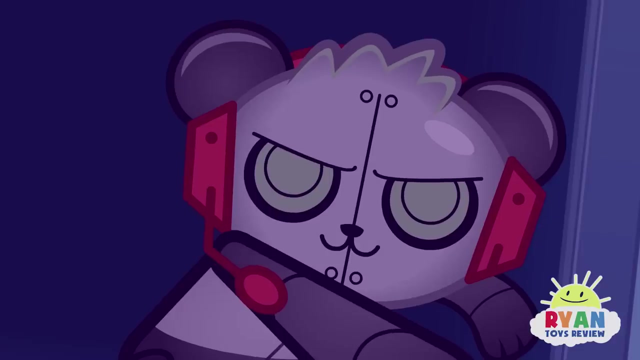 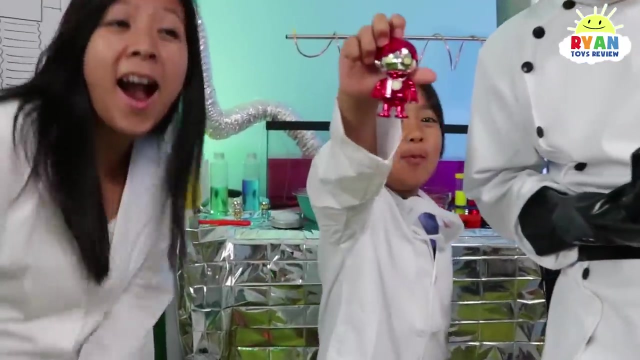 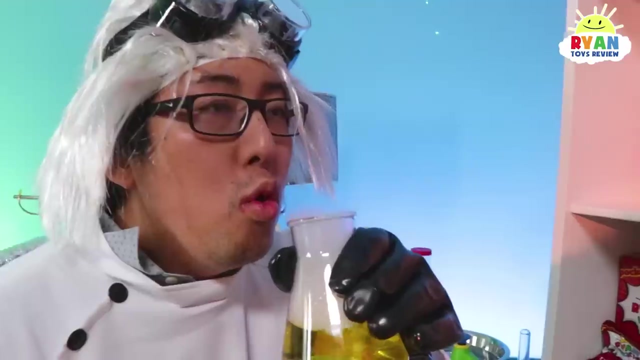 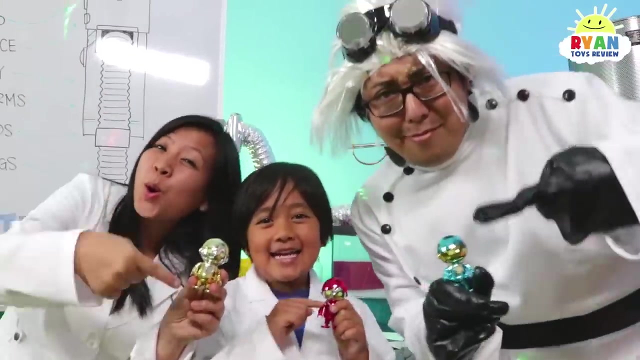 Oh, Oh, Oh, Oh, Oh, Oh. Here we go. combat failed, It's showtime. Hey guys, What should we do today? I have an idea. Let's build a robot. I'm gonna build a robot. It's gonna be My best friend. I'm gonna build a robot. 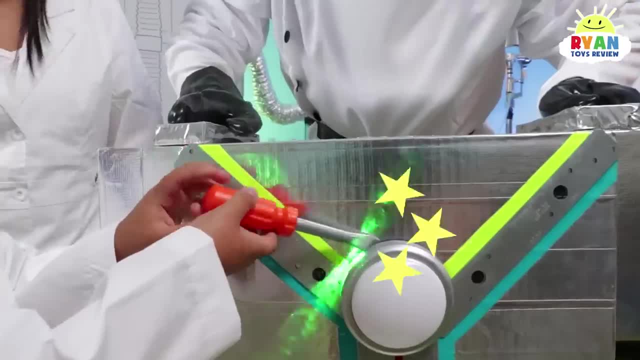 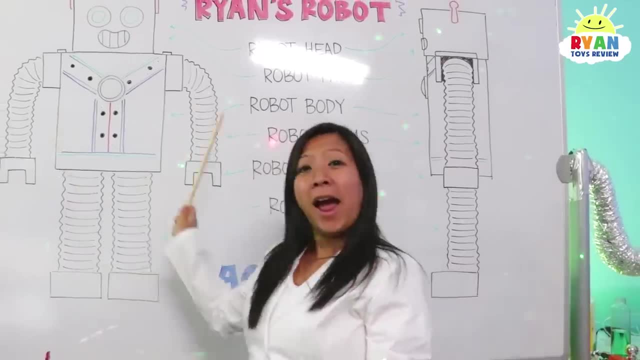 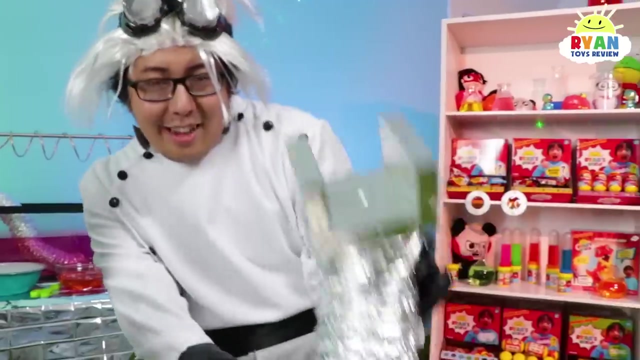 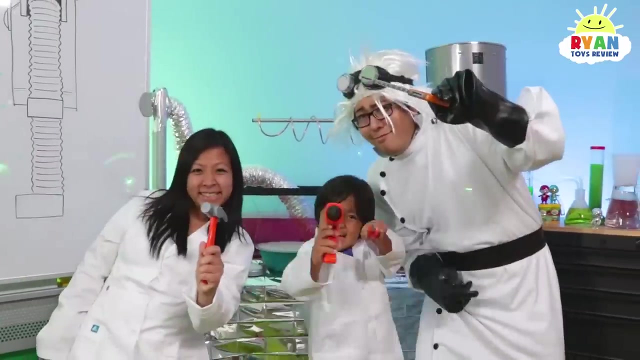 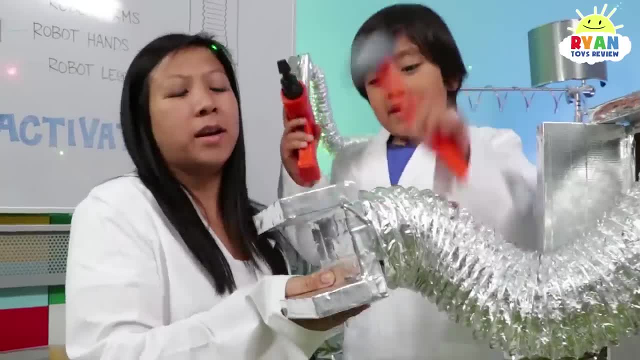 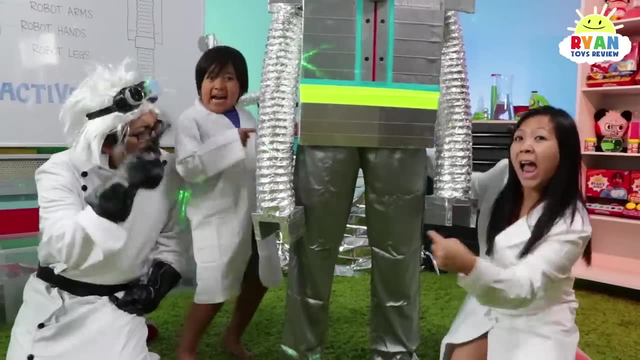 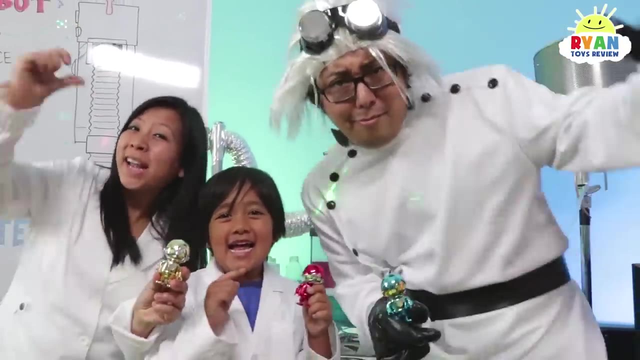 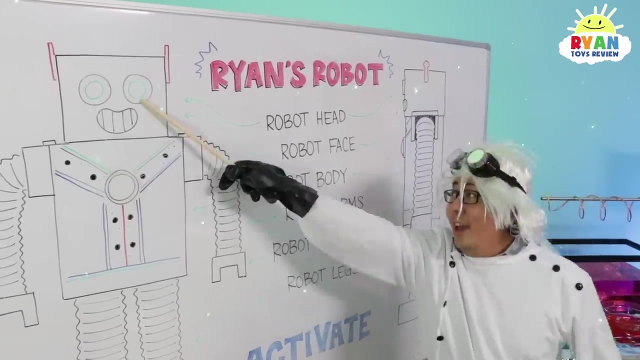 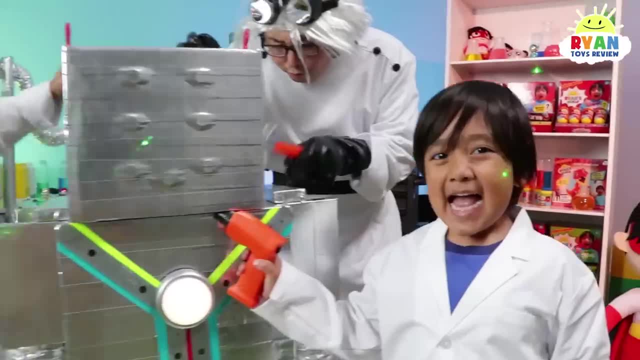 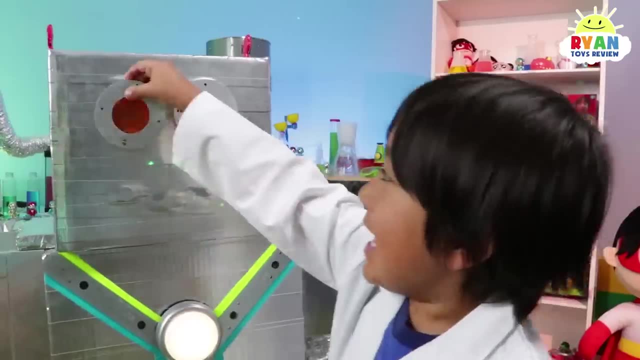 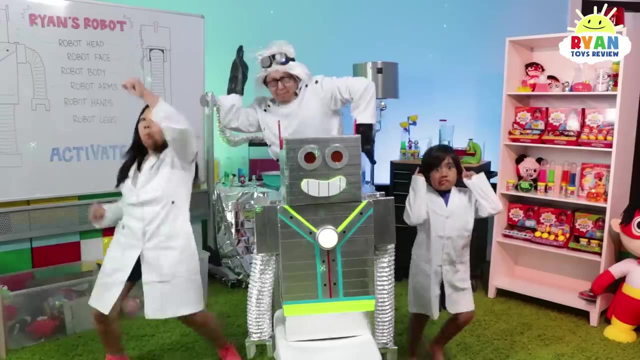 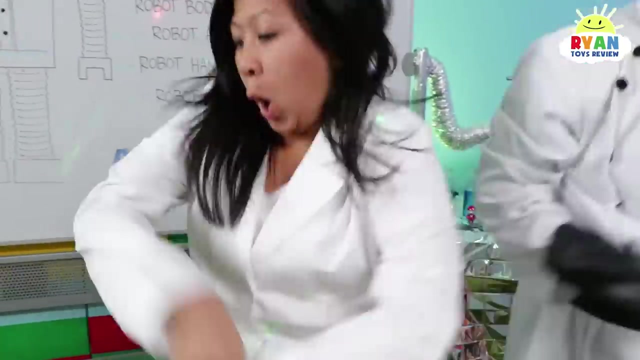 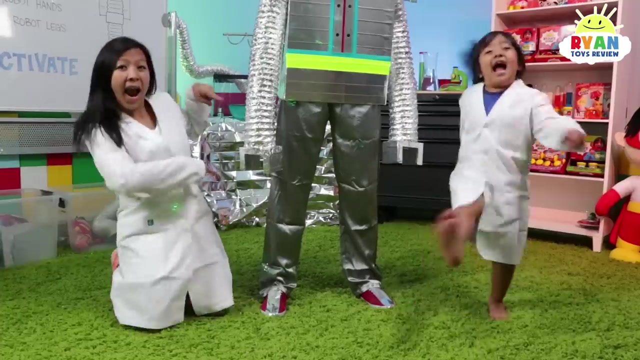 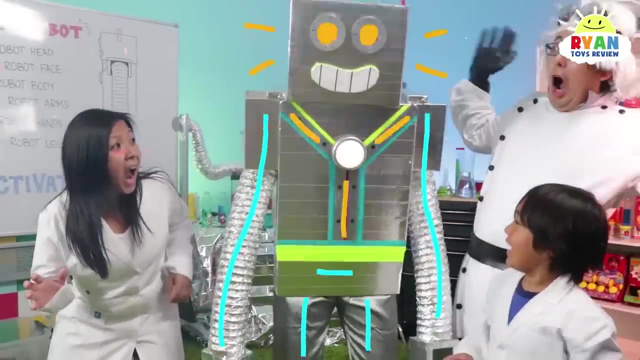